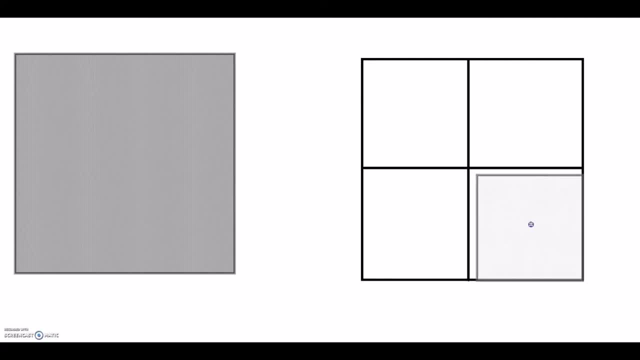 Well, I see these 1-by-1 squares, and I see 1,, 2,, 3,, 4 of these 1-by-1 squares on the checkerboard- I'm going to label this as a 1-by-1, and I see four of them. 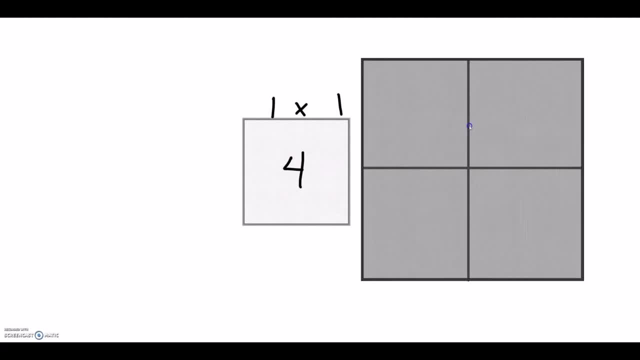 This large square right here is actually a 2-by-2.. This 2-by-2 square, and I only see one of them, so I'm going to go ahead and label this as a 2-by-2.. It's a 2-by-2, and there's only one of them. 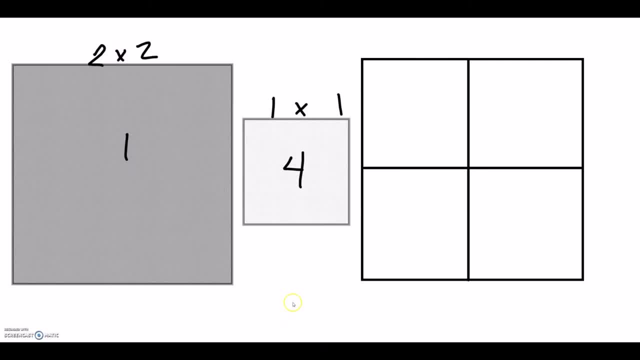 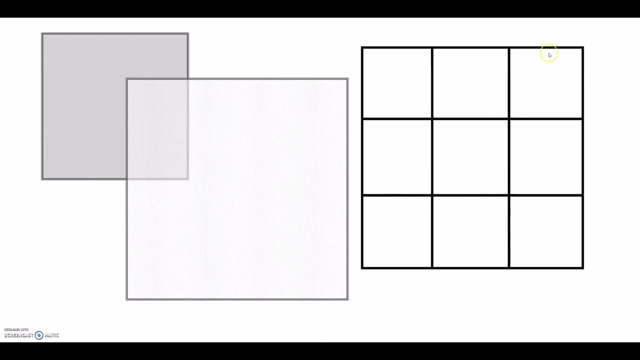 So all together on the checkerboard, this 2-by-2 checkerboard, we have four of the small squares plus one of the large squares, so a total of five squares on this 2-by-2 simplified checkerboard. And let's now step up to a 3-by-3 checkerboard like this one over here on the right. 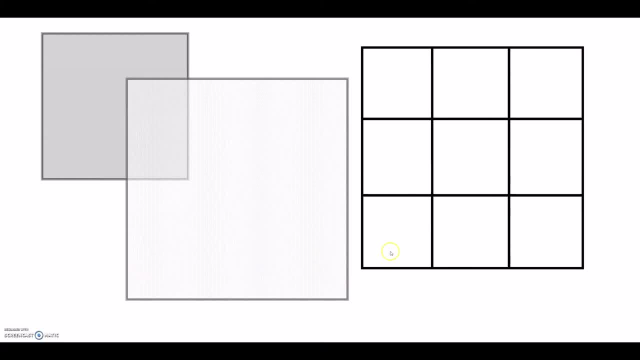 Now, I don't have the small squares on here, but we can fairly. We can fairly easily count that there's 1,, 2, 3, 4,, 5,, 6,, 7,, 8, 9 of the 1-by-1 squares. 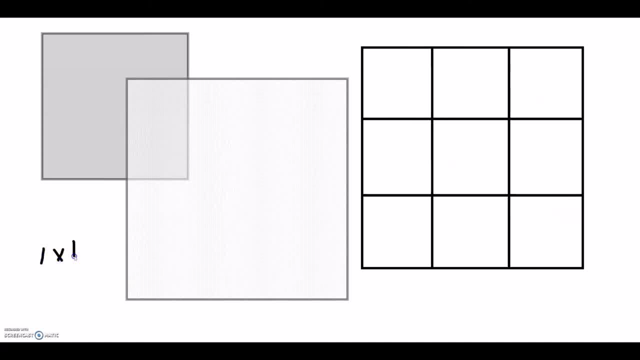 And I'm just out to the right or out to the left, going to put 1-by-1.. There are a total of 9 of those squares. Now this one right here represents our 2-by-2 squares and I definitely can see one. 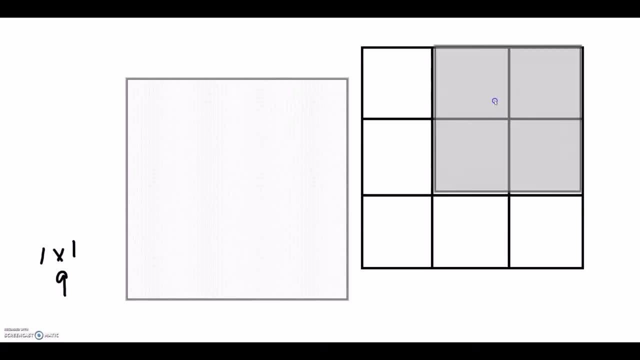 Then we have one here that overlaps 2,, 3, and 4.. There are four different ways We can do a 2-by-2 square, so I'm going to label this as 2-by-2, and there are four of those. 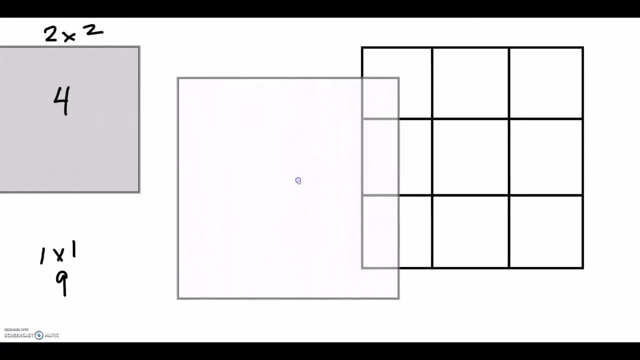 And this would represent our 3-by-3, and obviously there's only one 3-by-3 square, So let's label this as a 3-by-3, and there's one. So all together we have 9 plus 4 plus 1, which gives us what? 14 total squares in the 3-by-3 checkerboard. 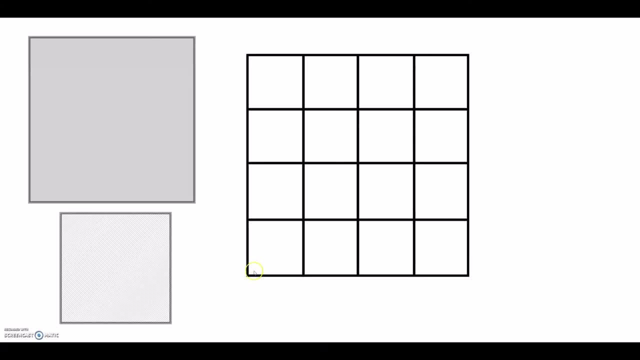 Okay, Step up to a 4-by-4 checkerboard like the one that we have here on the right, And in a 4-by-4 checkerboard we're going to have 4 times 4, which is 16 of the small squares. 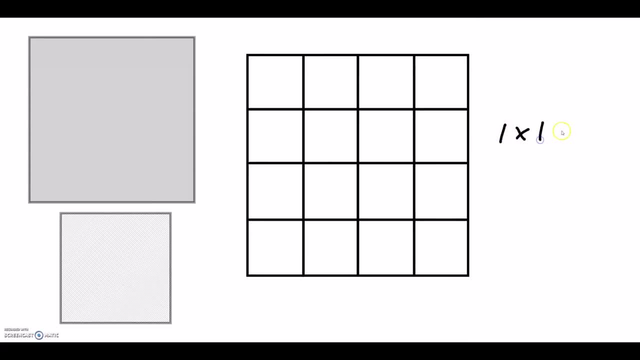 Those small squares are the 1-by-1 squares and there were 16 of them. I don't want to put an equal sign here, so I'll put a dash, because 1 times 1 doesn't equal 16, but there are 16 of the 1-by-1 squares. 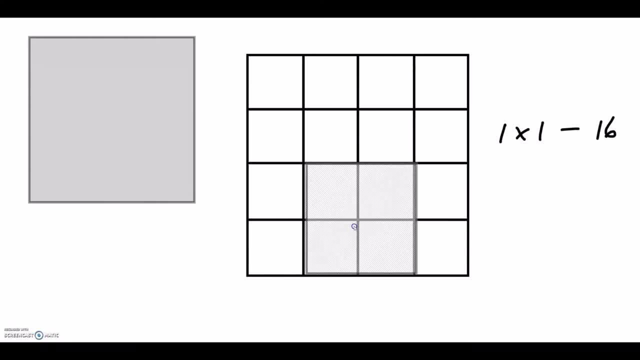 Here are the 2-by-2 squares. I see 1,, 2,, 3.. 4,, 5,, 6,, 7,, 8,, 9 of the 2-by-2 squares. I'll put this out to the right as well. 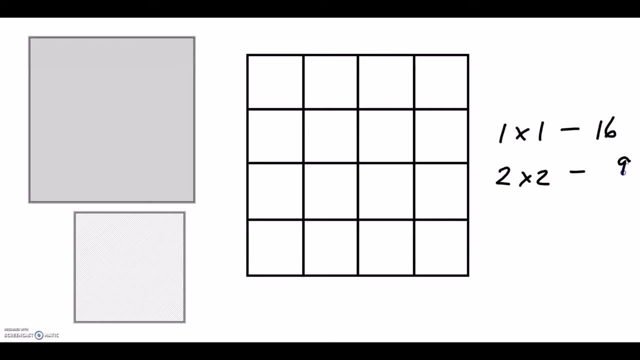 So 2-by-2 squares. we had 9 of them, And here's your 3-by-3 squares: 1,, 2,, 3,, 4 of them. I'll write that out to the right as well. 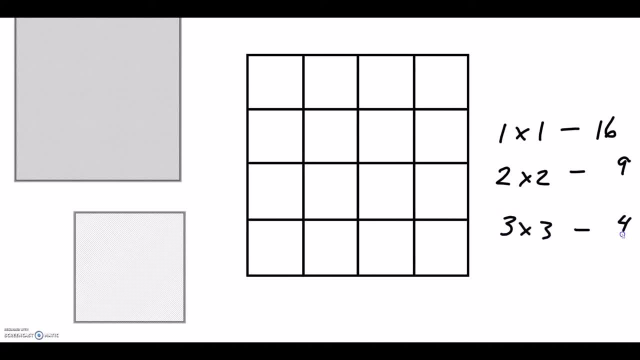 3-by-3,. we had just 4 of them And I don't have a 4-by-4 drawing. I don't have one on here, but we can see that the 4-by-4, there's only going to be 1,. 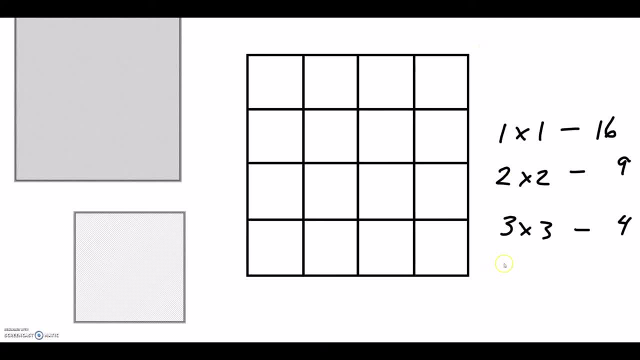 because we only have one big 4-by-4 square. So I'll put that down here: at the bottom: 4-by-4, we only have one of them. So all together 16 plus 9 plus 4 plus 1.. 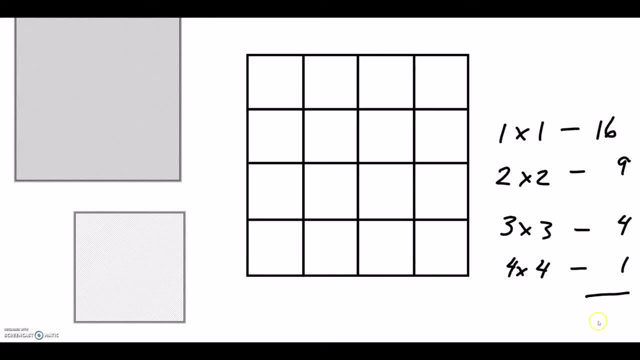 16 plus 9 is 25 plus 4 plus 1.. That's going to be what 30 squares total on our 4-by-4.. If you're looking carefully, you can kind of already see some patterns that are developing. 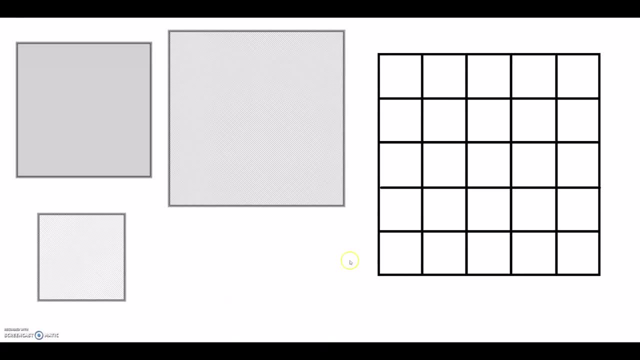 And here is our 5-by-5 checkerboard. Of course, on our 5-by-5 checkerboard there will be 5 times 5 of the 1-by-1 squares, So that will be 25 of the 1-by-1 squares. 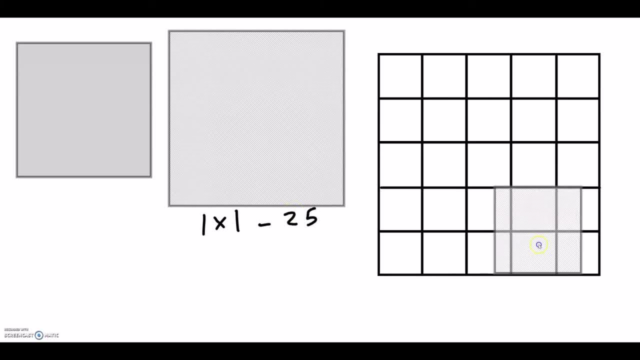 Here are our 2-by-2s: 1,, 2,, 3,, 4,, 5,, 6,, 7,, 8,, 9,, 10,, 11,, 12,, 13,, 14,, 15, 16.. 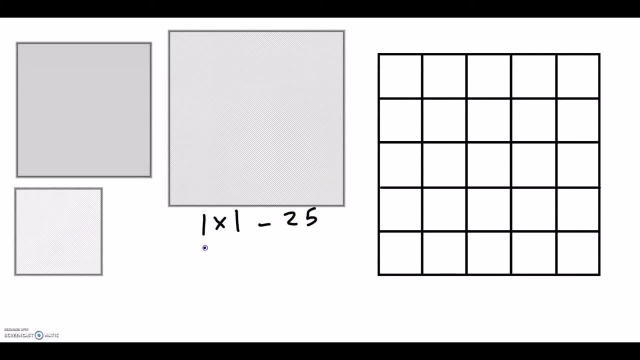 I'm hoping you're now starting to see a pattern And if you do see a pattern, try to guess. before I show you how many 3-by-3 squares there are, try to guess how many you think there will be. Here's a 3-by-3.. 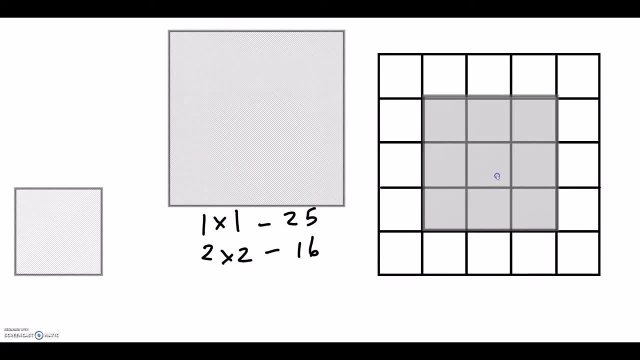 1,, 2,, 3,, 4,, 5,, 6,, 7,, 8, 9.. Did you get 9?? If you got 9, then you probably can guess how many of the 4-by-4 squares there will be. 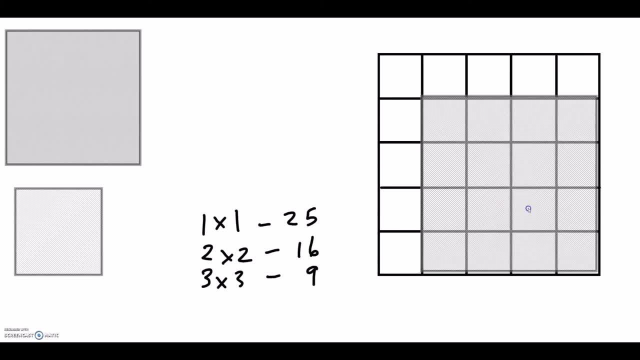 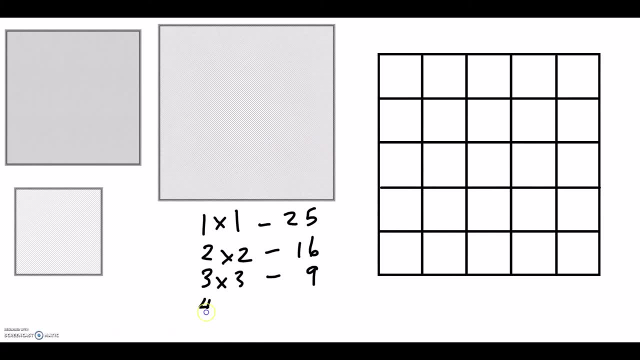 See if you can guess that There's 1., 2., 3., 4., And then, of course, of the 5-by-5s there's only going to be 1.. So the 4-by-4, we got 4.. 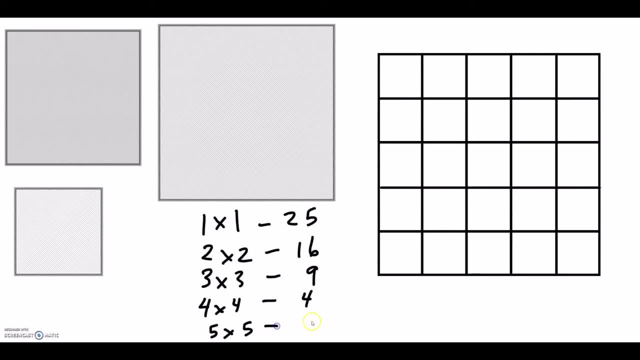 And the 5-by-5, there is just 1.. So what we have here is we have 30 plus 25.. All together is 55 squares on the 5-by-5 checkerboard. Hopefully you're now really seeing a pattern. 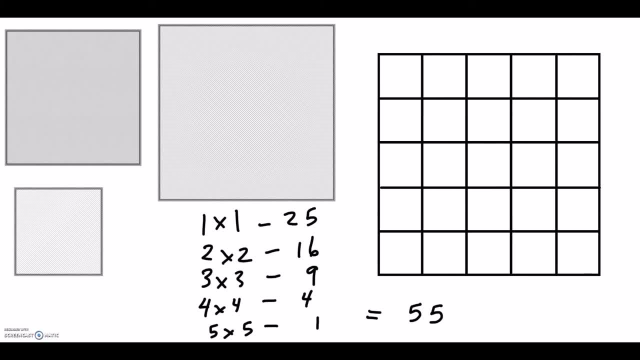 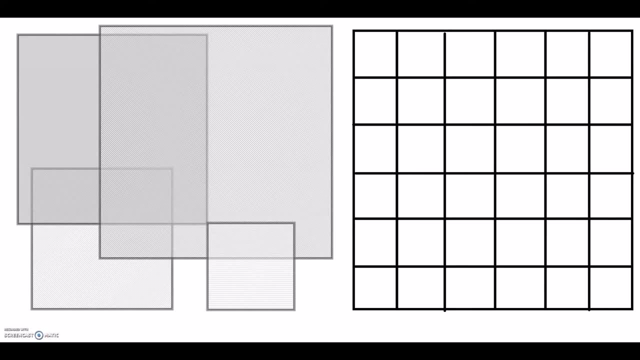 But you could now apply to the 6-by-6 checkerboard. Before I show you the 6-by-6 checkerboard, see if you can do it on your own. Think about the pattern that you've seen over the last several steps that we've done. 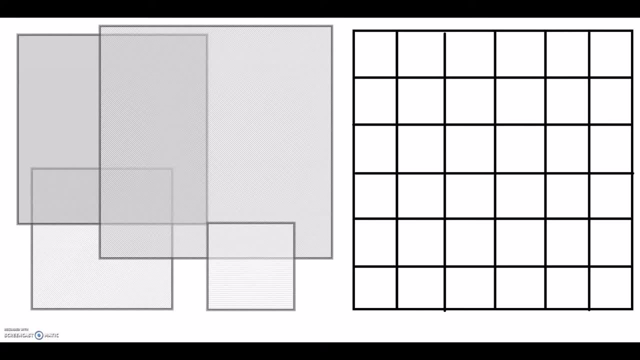 and see if you can extend that pattern by one additional step. Obviously, in this 6-by-6 checkerboard we're going to have 36 of the small squares, the 1-by-1 squares, And then, if we take these 2-by-2 squares, we have 1,, 2,, 3,, 4,, 5,, 6,, 7,, 8,, 9,, 10,, 11,, 12,, 13,, 14,, 15,, 16,, 17,, 18,, 19,, 20,. 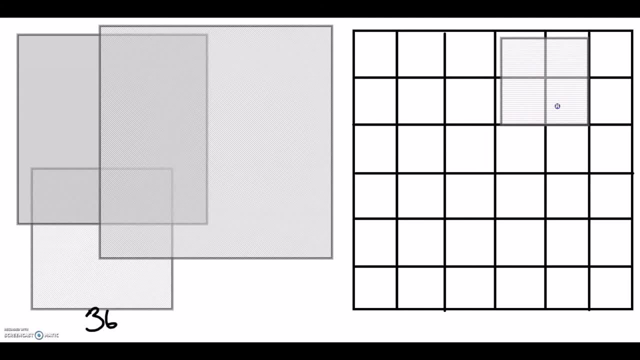 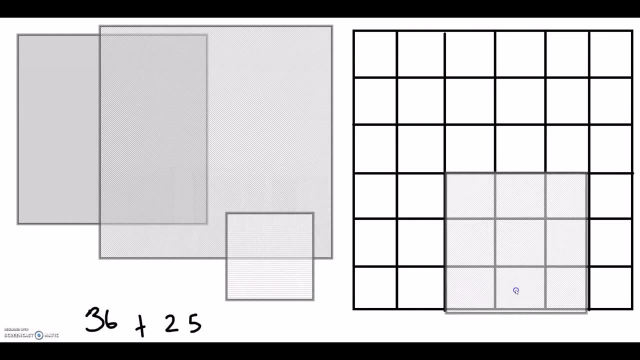 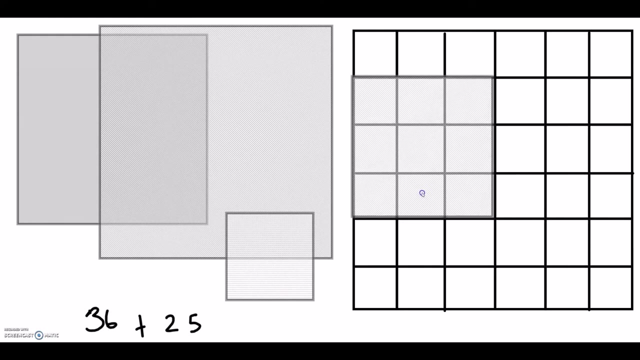 21,, 22,, 23,, 24,, 25 of the 2-by-2s. So let's do that. So let's add that The 3-by-3s 1, 2,, 3,, 4,, 5,, 6,, 7,, 8,, 9,, 10,, 11,, 12,, 13,, 14,, 15,, 16.. 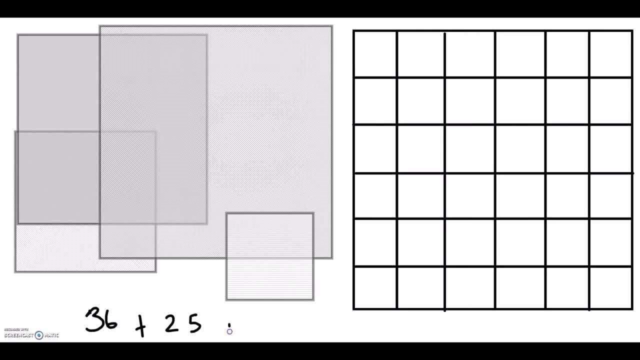 So 16 of the 3-by-3s. I bet you can predict how many 4-by-4s there will be. Here are our 4-by-4s: 1, 2, 3, 4,, 5,, 6,, 7,, 8, 9.. 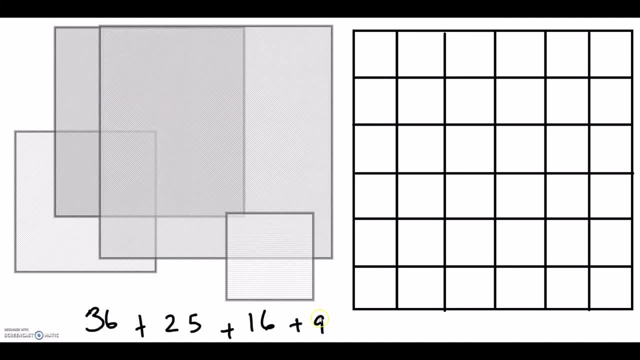 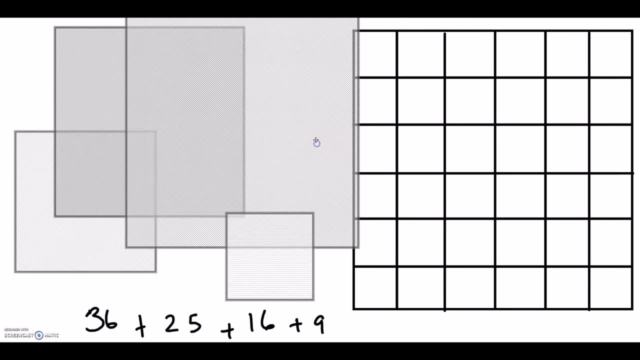 And I certainly bet you can predict how many of the 5-by-5s: 1,, 2,, 3,, 4.. And then, of course, we know that we have a 4-by-5.. So we know that we have a 4-by-5.